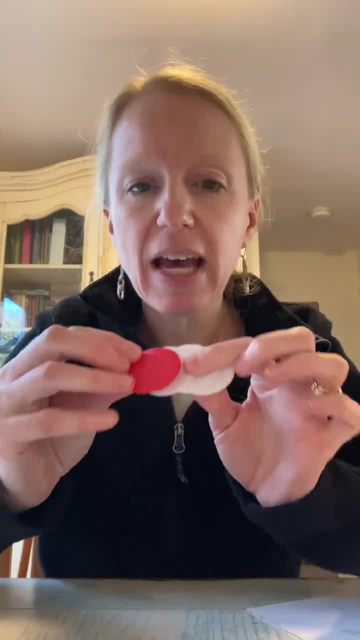 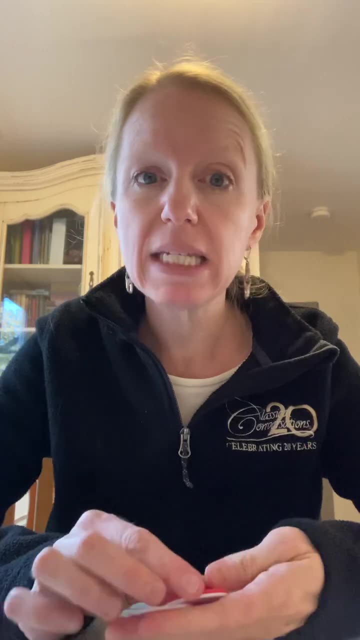 for our purposes. And so if I have one red, three white poker chips in my hand and you want to roll the dice, you're going to roll the dice And you're going to roll the dice and you want the red one. What is the probability that if I have this, you're going to draw the red? 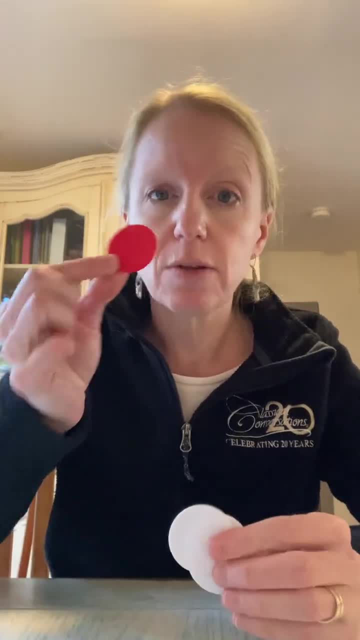 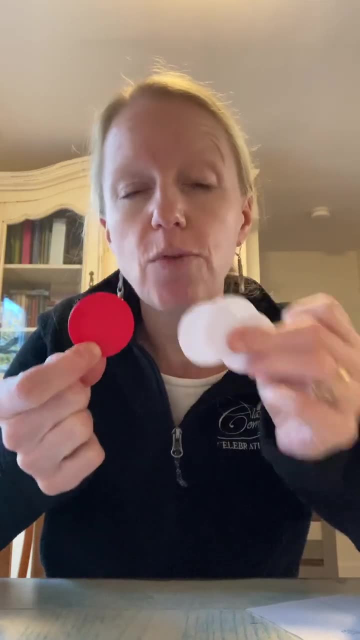 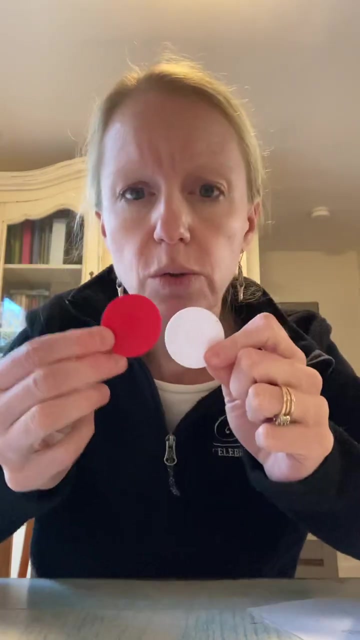 one. Well, our desired outcome is red out of our total possible outcomes, which is four. So we have one in four chance or probability of getting a red poker chip. Now you might say, well, there's only two colors, just like there's only two colors in the deck of cards. That's true, There's only 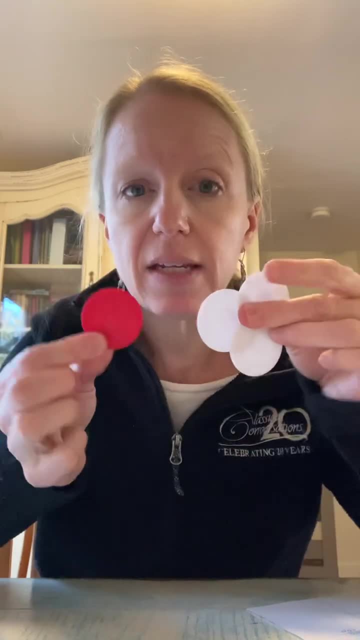 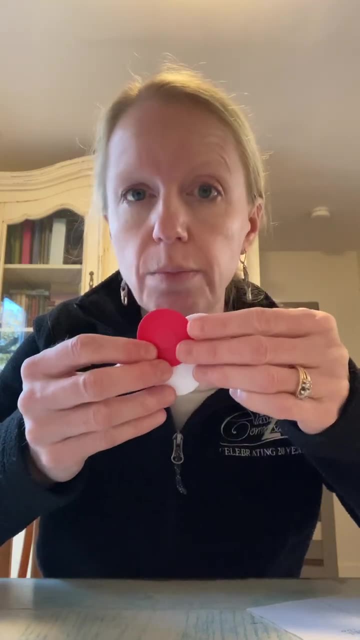 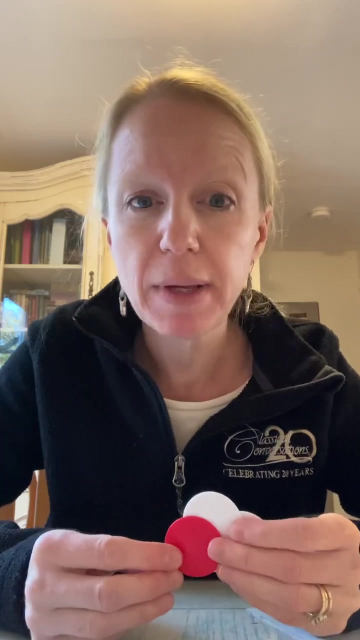 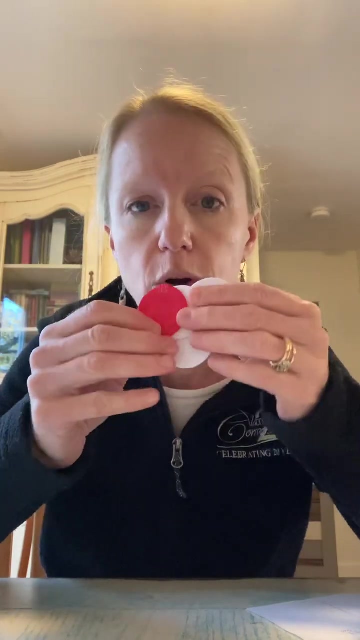 two colors, but there is not an even number of possible outcomes, And so it gets a little more complex when you have not an even distribution of things, like we did last week. So again, probability is desired outcome over total possible outcomes, So one out of four chips. 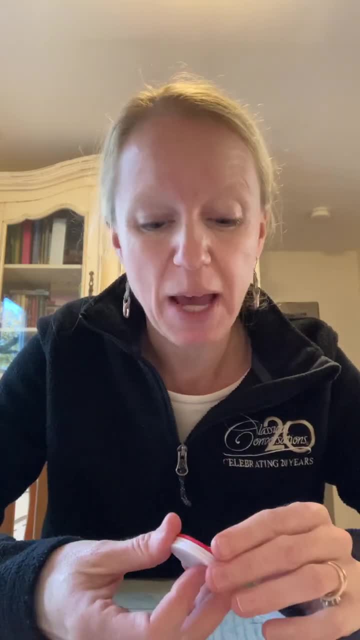 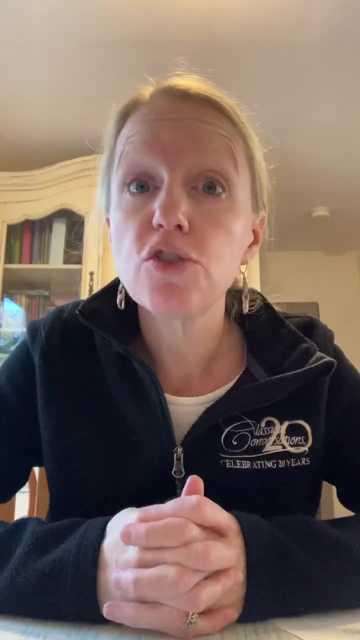 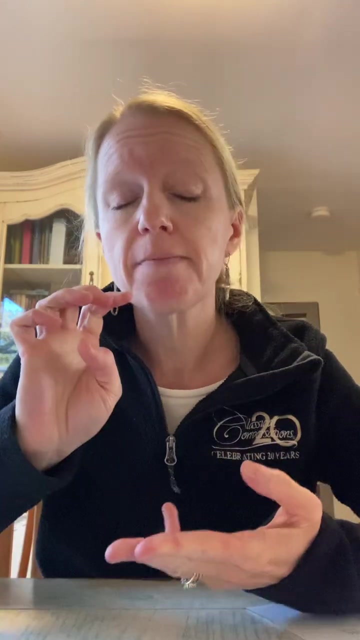 would be how you decipher that, And that's kind of starting in with that to kind of get this concept of an equal or an even distribution of possible outcomes. So we reviewed the definition, we reviewed why we study probability, We talked about a little bit more deeper understanding of how to acknowledge 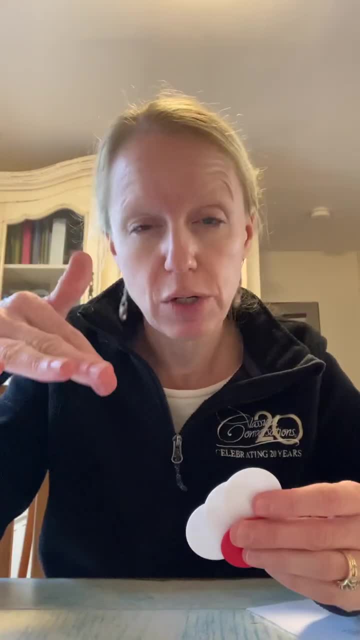 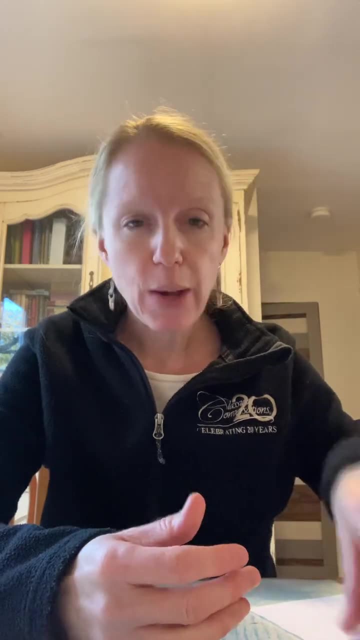 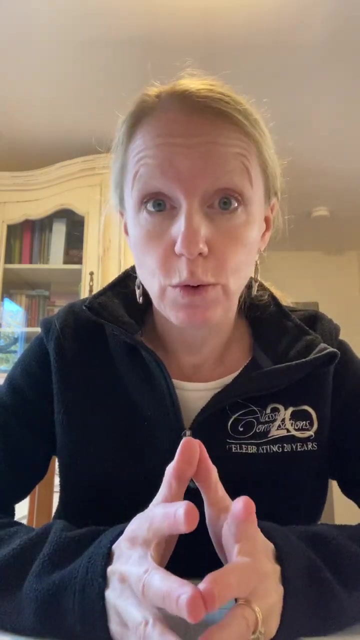 probability, again total or desired outcome over total outcomes. And then we're going to introduce new grammar today called sampling. So a sample that we're going to use is called sampling. The official definition would be a representative part of a statistical group whose properties are: 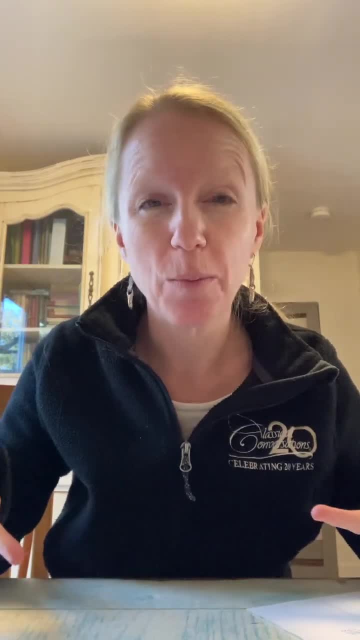 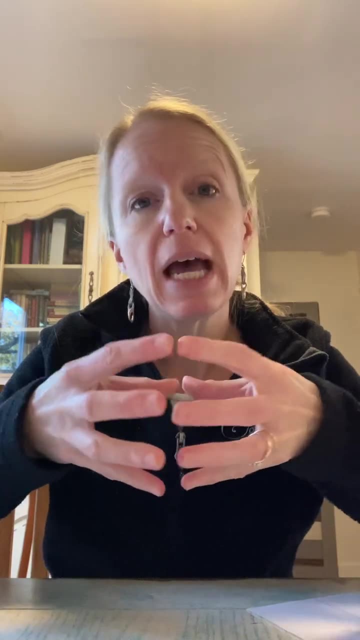 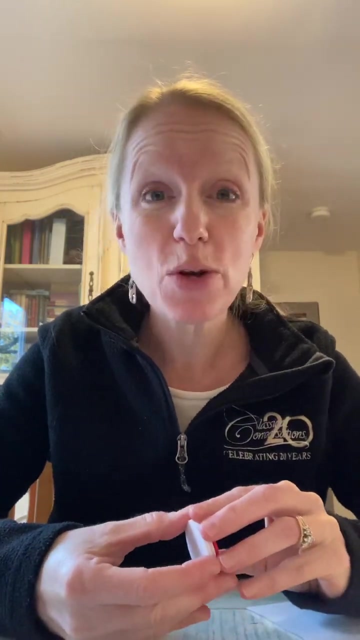 studied to gain information about the larger whole. So basically it's studying a small group or a portion of a group trying to find information about a larger whole. So if we were to study plankton in the ocean, there's no way a marine biologist could study all the plankton in the 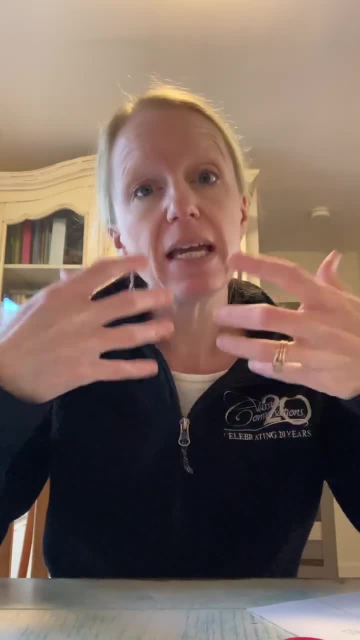 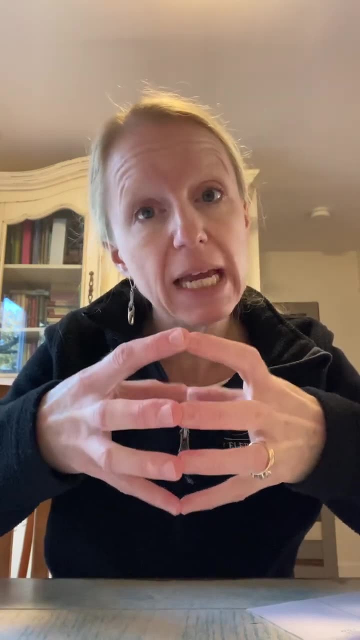 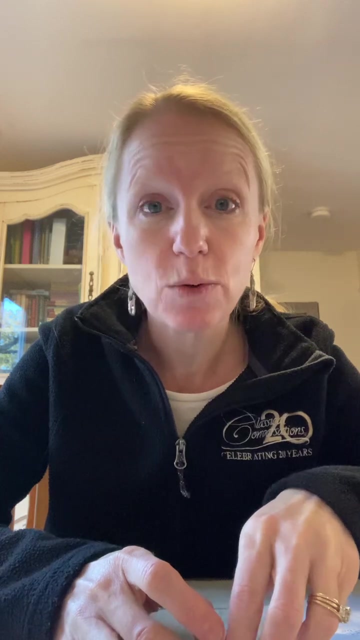 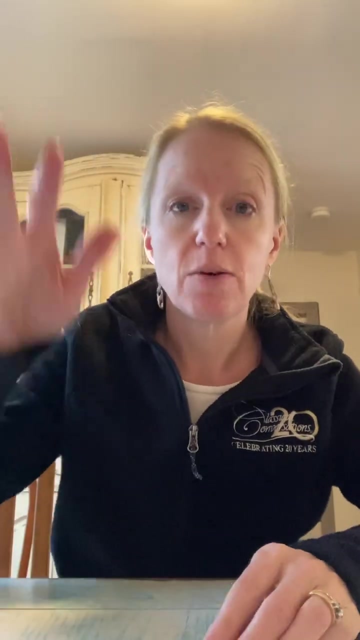 ocean So they might take a grouping and make probabilities based on that small group of plankton in a certain region of the world. I would do some sampling questions in the classroom. So, okay, of our eight or nine kids, how many of you like chocolate, ice cream? You know? raise your hand. 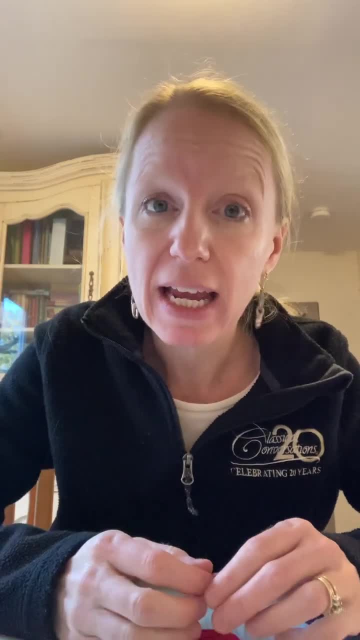 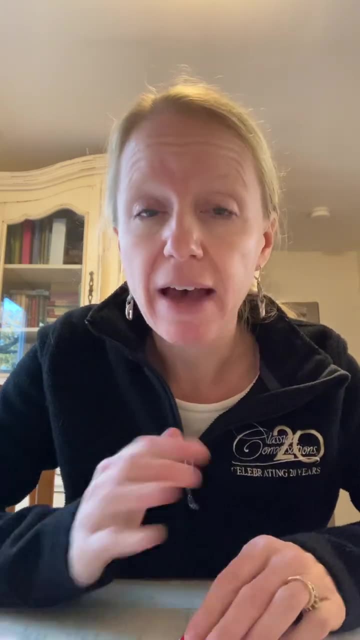 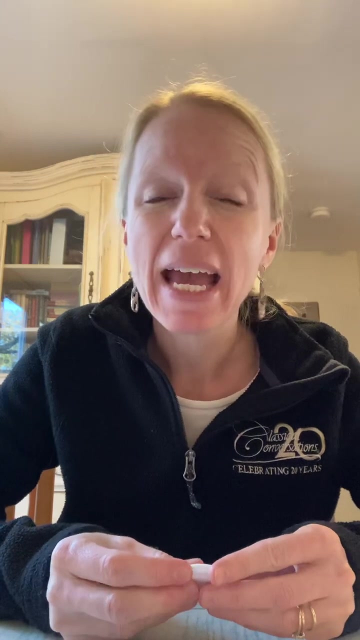 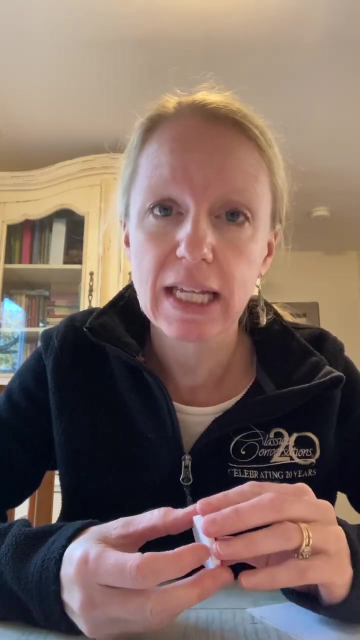 Well, if four out of the eight like chocolate ice cream, you could make an assumption that possibly about half of the children in the same age group as them across the world or across our nation like chocolate ice cream, And so you could do a sample question of how many of you in this classroom have more than one sibling. And again, 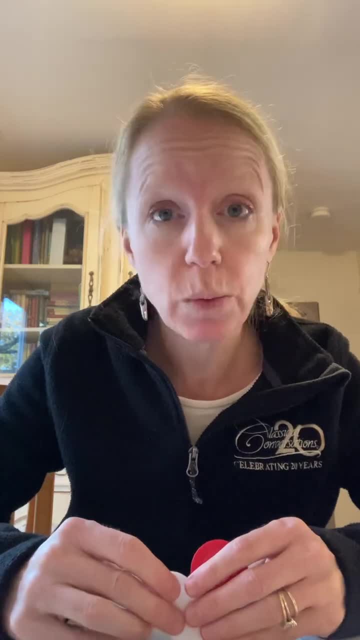 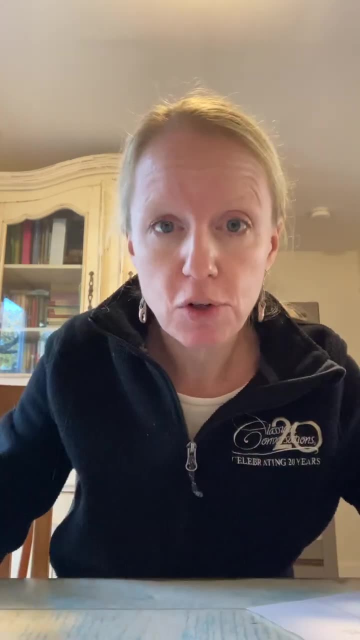 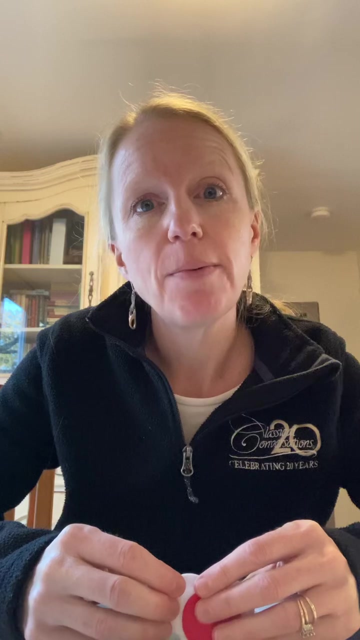 so out of the eight kids, if only two out of the eight kids have more than one sibling, then you might make an assumption that two out of eight or one out of four kids in that age bracket have more than one sibling. And so you start to get an idea of taking 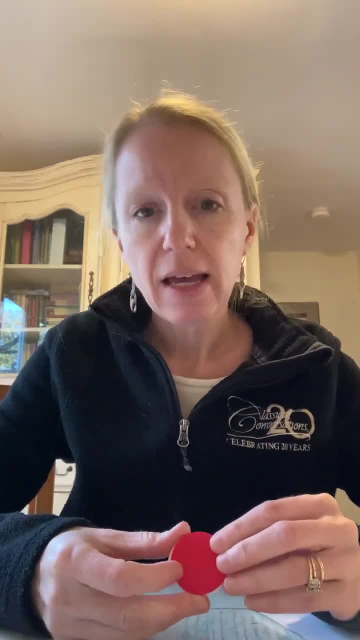 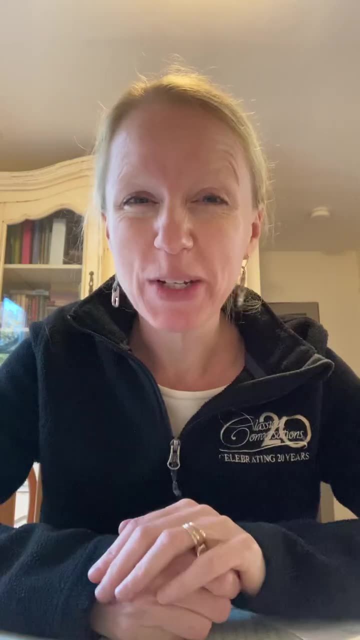 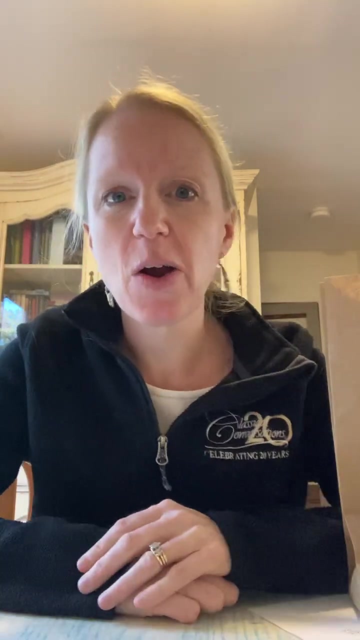 what a sample is. So today we are going to do a sampling experiment And to do this, we're using those poker tips and we're going to put them in a bag, and we're going to put them in a bag, and we're going to put them in a lunch bag, and then we're going to document our results. So we want to know. 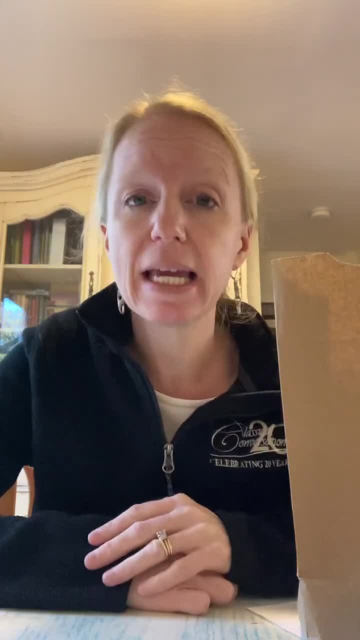 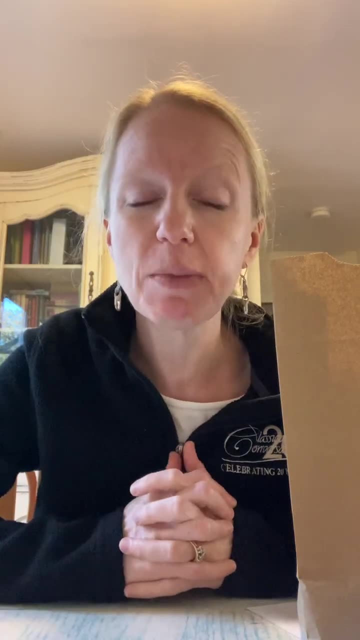 in this bag I have red, white and blue chips, but I don't know exactly. I do, But for your purposes as a tutor and doing the experiment you're going to say, I don't know exactly how many of each. we. 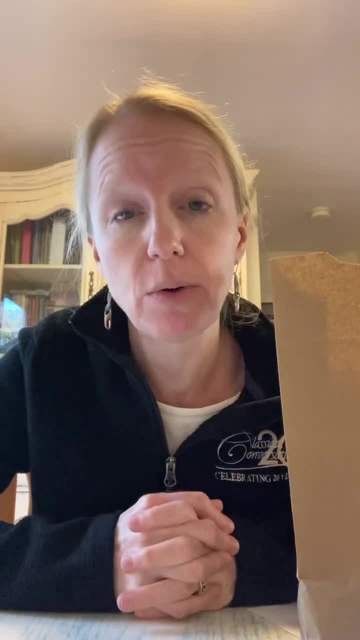 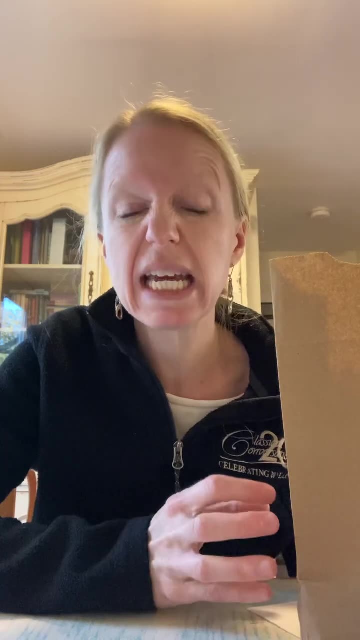 have, but I do know there is not an equal number of each, And so we're going to take a sample. we have 100 chips total. We're going to take a sample. We're not going to study all 100, but we're. 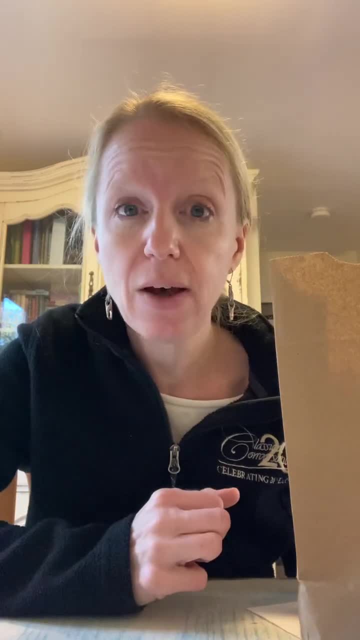 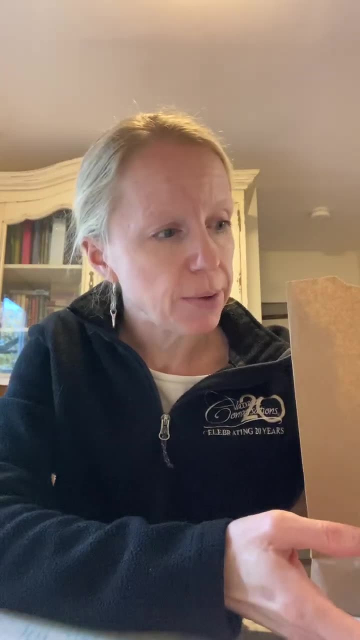 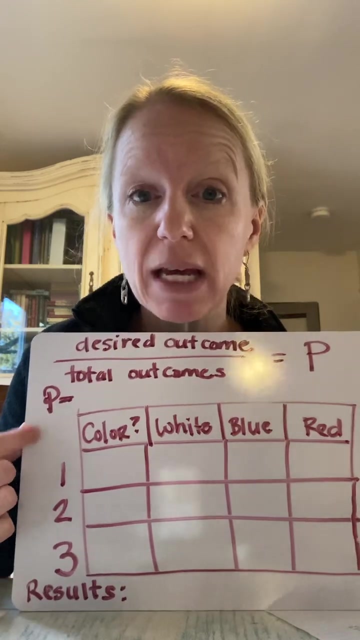 going to do a sample to see if we can get statistically about the probability of each chip, of drawing each chip each time you do it. So, to do this, you're going to make a chart on your boards. I'm not giving you pre-printed because it'll be better, bigger. So you're going to do this with 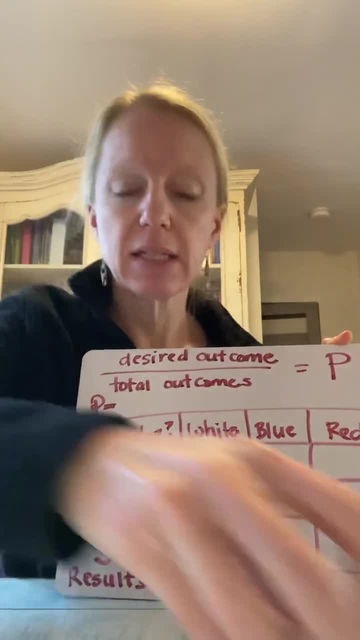 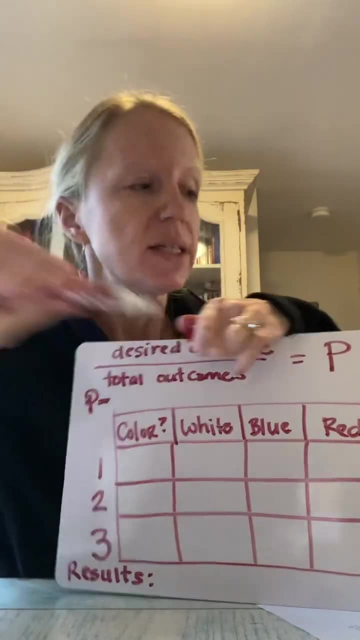 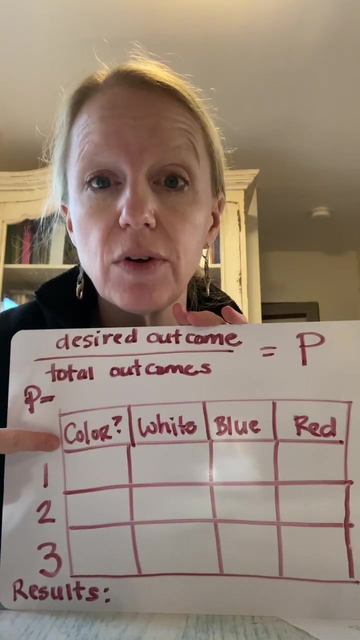 your kids. I'm going to go through it a couple times because it's a little confusing looking at it in our curriculum guide- At least it was for me- And so you kind of walk through it So out of my bag here. So this is what your chart is going to look like. You're going to have color in the first. 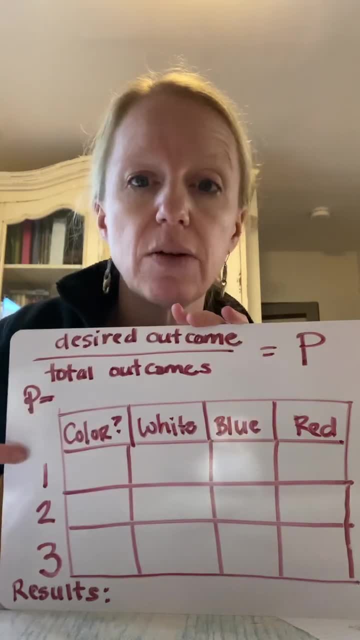 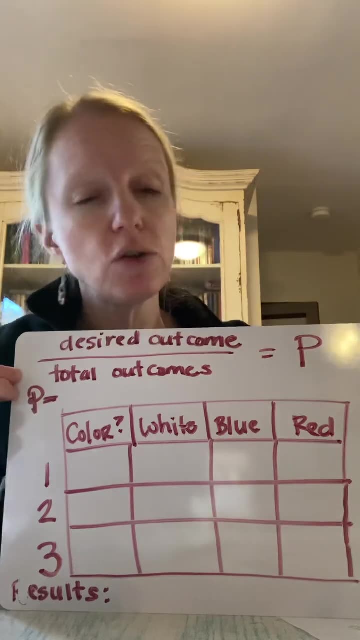 one. Then you're going to have white, blue and red And then on this side you're going to write just the number of times you do it. I want you to go around the room, have each student draw a chip to use. 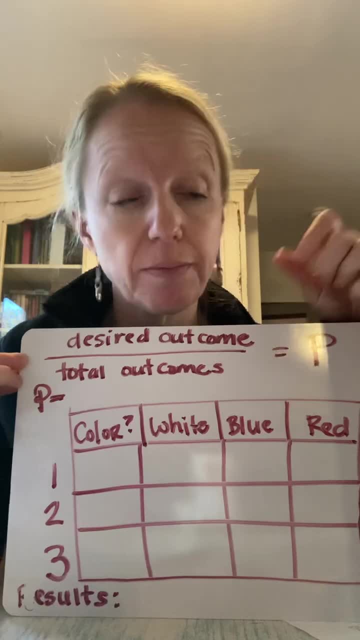 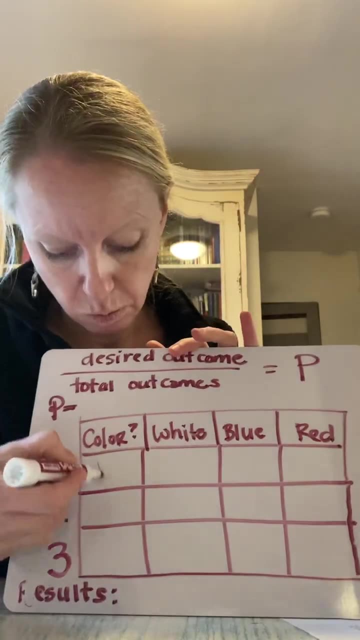 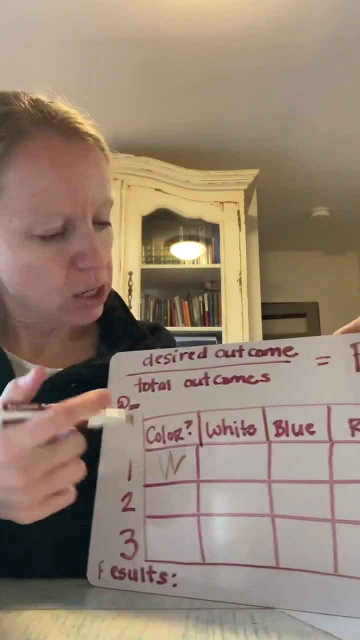 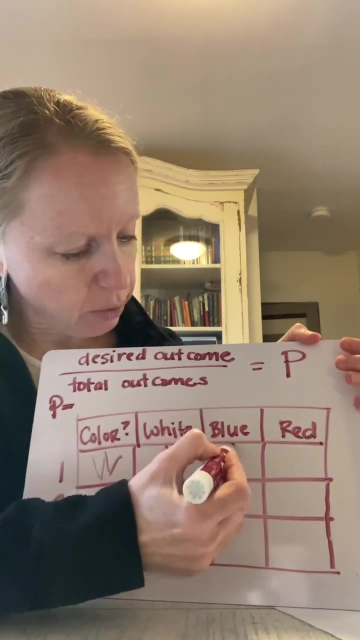 So I'm going to say I drew out a white, So I'm going to put white here, W for there. Now you kind of each row, you're going to make kind of a results of each one. So of the white I did one, I got one white out of one tries. Blue: I've gotten zero out of one try, And red: I've gotten zero out of one try. 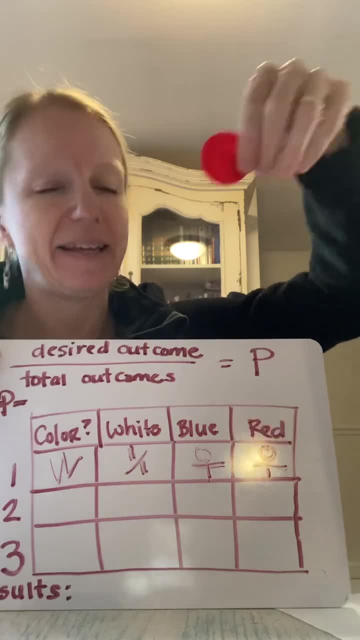 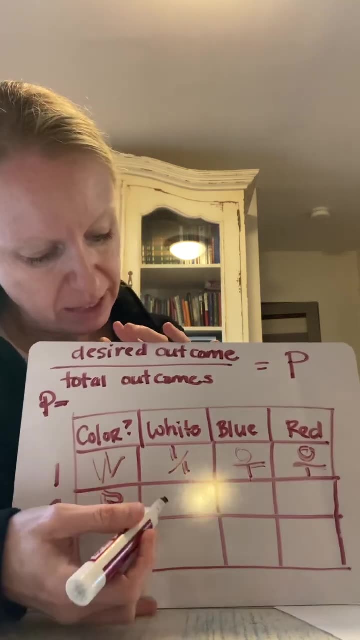 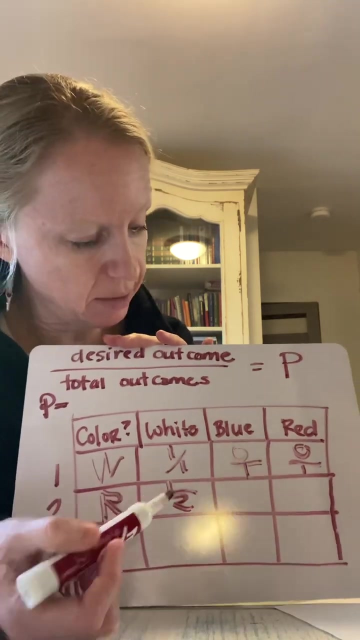 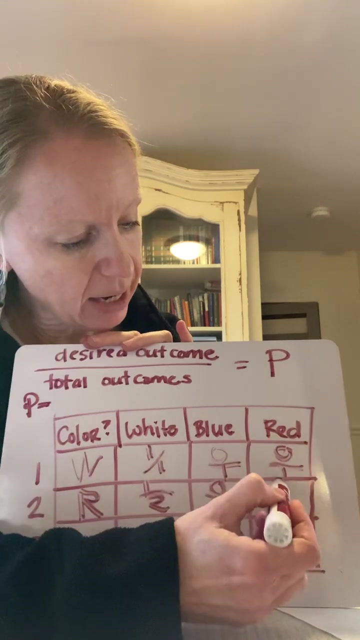 So I'm going to draw the next one. Red: All right, so I got red. So now with I'm going to put my R for red And then white: I still got one, But now I have two tries, So I've gotten one out of two tries. Blue: I still have zero, But now I have two tries, So one out of two Red: I now have one out of two. 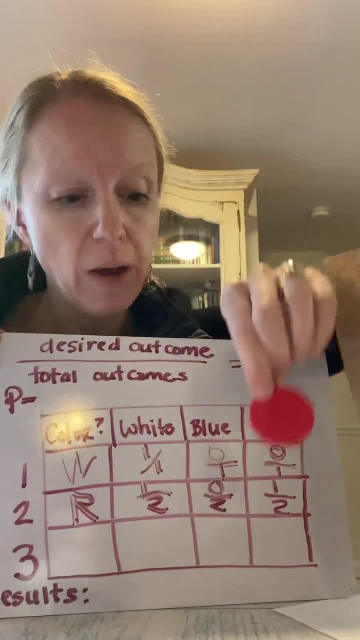 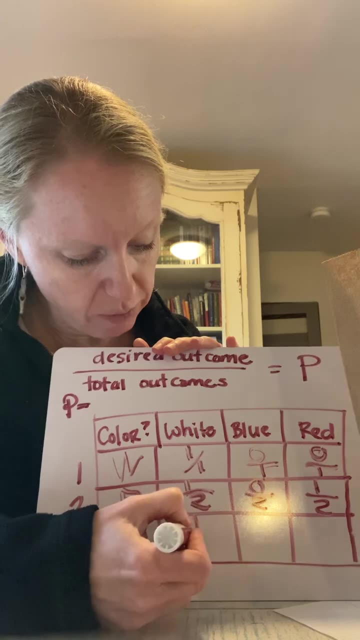 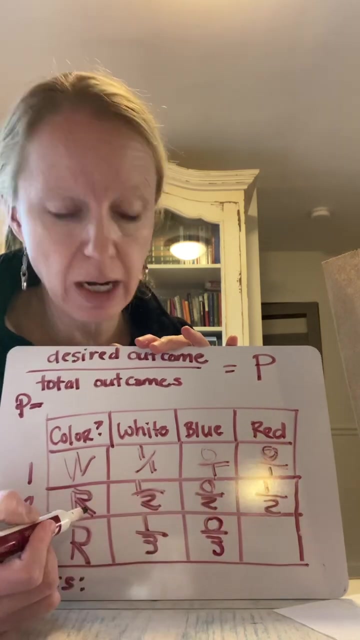 Okay, I get another red. Okay, so I put my red, My white- I still had the one from the first time, So I have one, And now it's out of three tries. The blue- poor blue here- zero out of three tries- And the red: now I have two out of three tries. 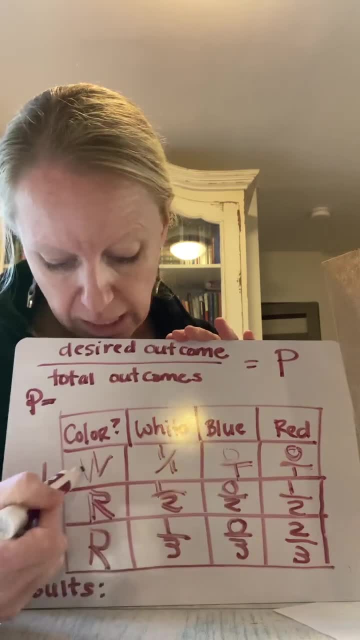 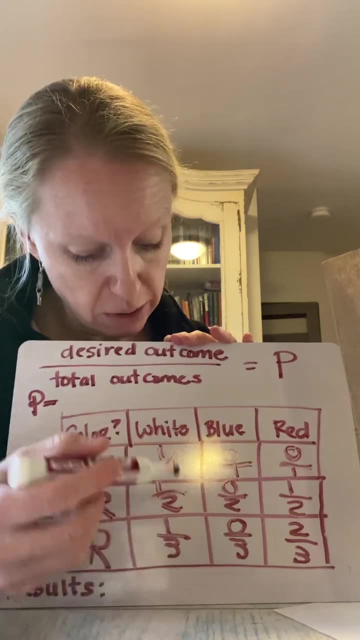 And so you continue on each time just counting how many you've gotten of that one, And then the bottom number is the total. So this is your desired outcome over your total outcomes. on the bottom, the total number of tries that you've done it. 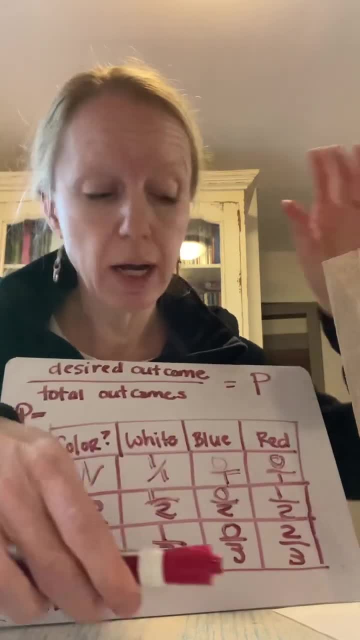 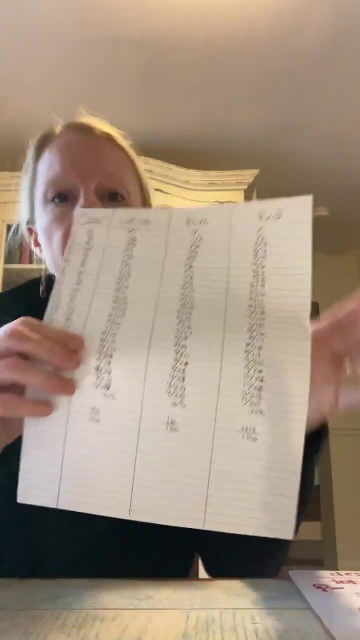 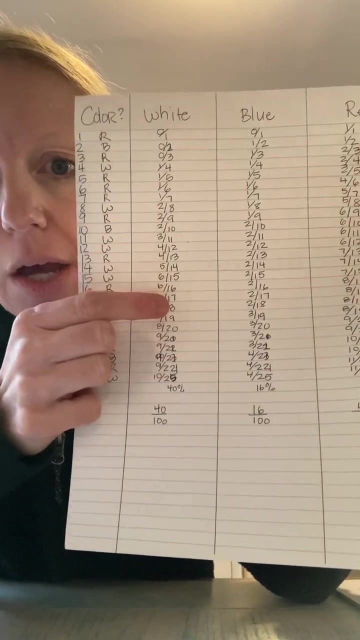 And then you're going to keep going for 25 tries. Now I have done this, this particular one, And just to give you an idea of what it might look like, And so you can see each time I have the number of times that it was done over the total number. 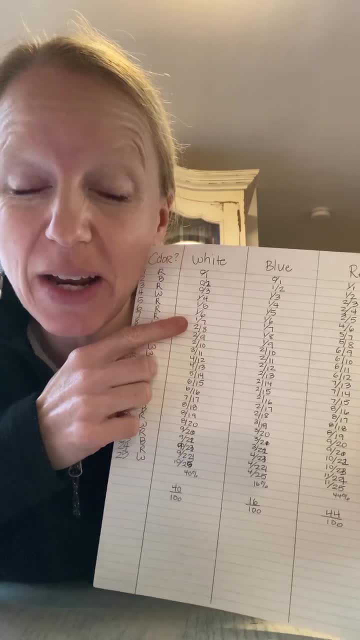 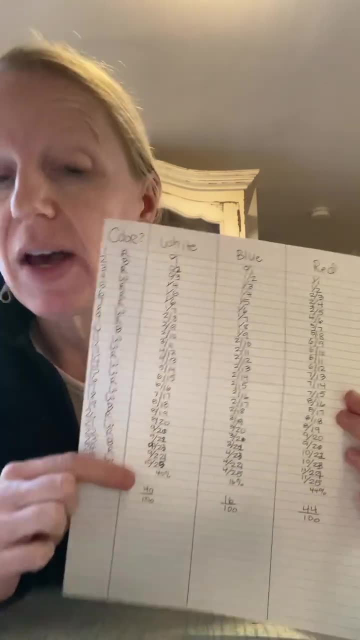 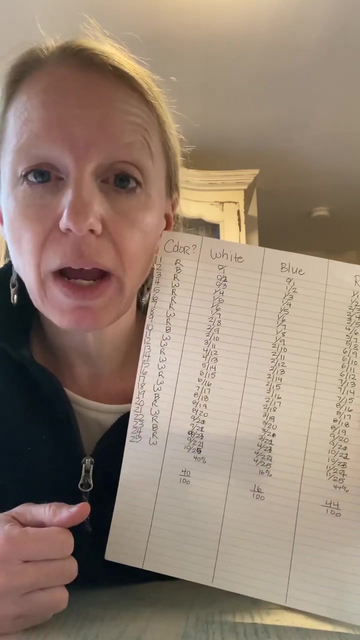 So the top number is the desired outcome of that color And then the bottom is the total number draws. that we've done By 25 draws. you should be pretty close to getting an estimated probability of how many are in each there, Or what would be your likelihood probability of drawing that color. 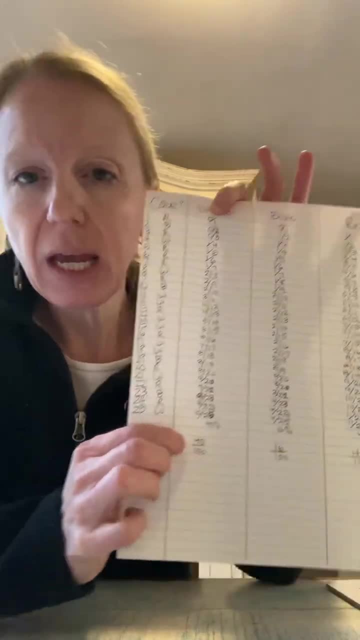 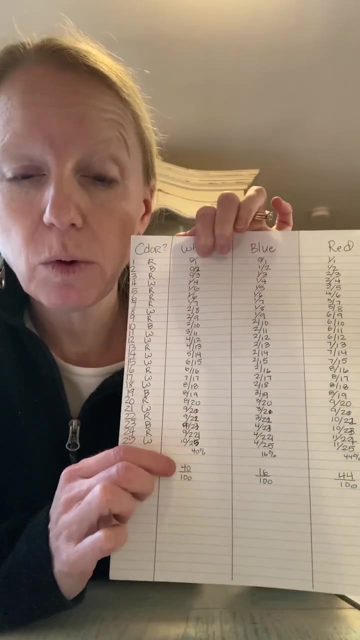 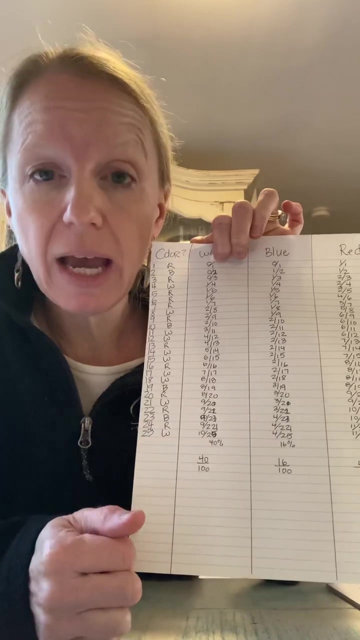 And so I did my white. I got to where I had. a total of 10 out of 25 were red draws, And so that gave me about a 40% times 100, 40 out of 100. It would estimate. that's how many are in my bag. 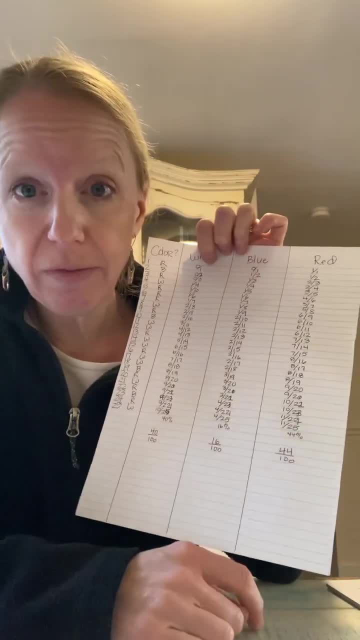 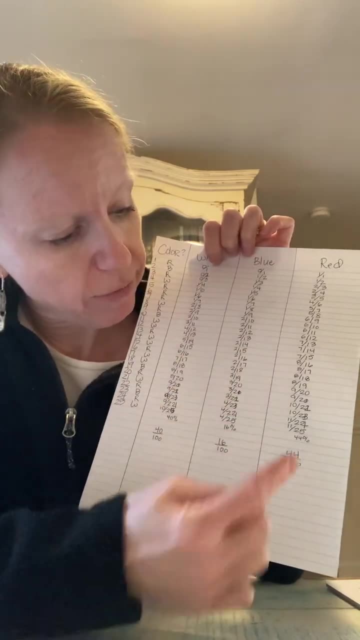 Blue, I had a total of 4 out of 25 draws. That's 16%, So 16 over 100.. And then the red: 44%, and that's 44 over 100.. The actual number that I had in there is pretty close. 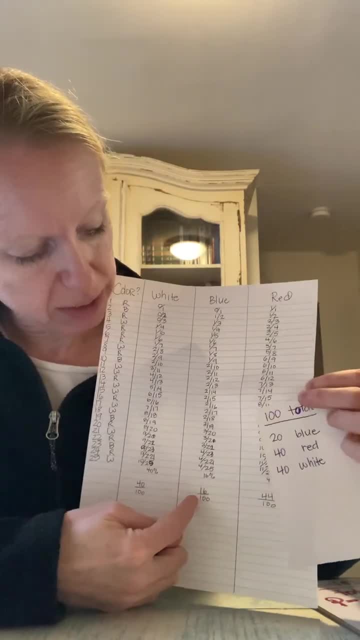 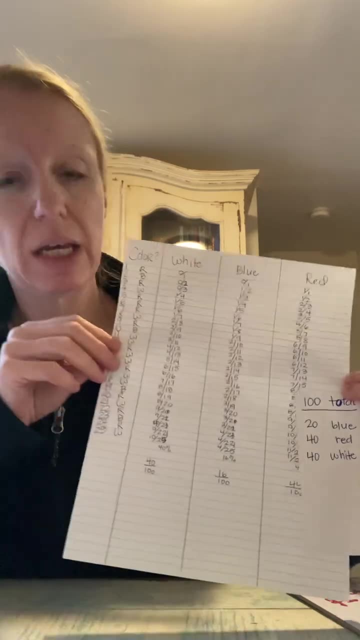 So, blue, I had 20, and again the results were 16 out of 100.. Red, I had 40,, and that was 40 out of 100.. And white, I also had 40, and I had 44 out of 100. 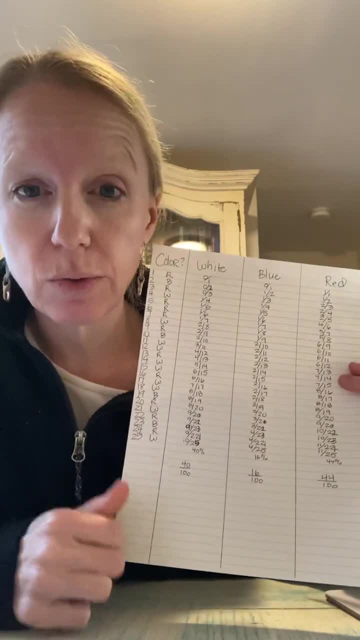 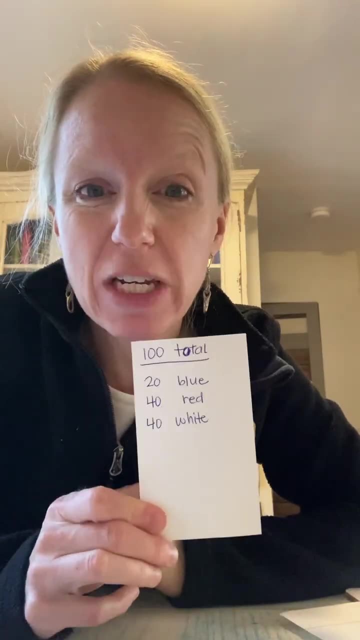 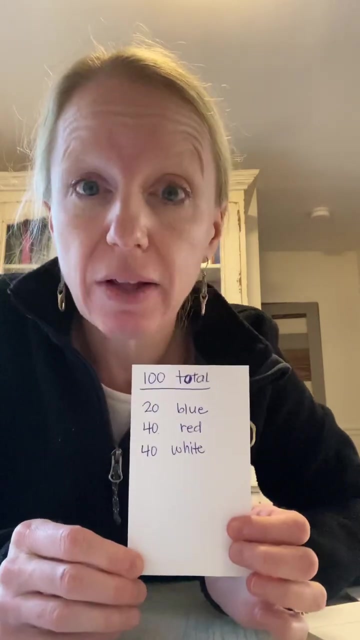 So doing the 25 tries was pretty close to the actual number of each color In your bag. tutors, you will have your little cheat sheet to know at the end to be able to compare your results to the actual number of each color in your bag. 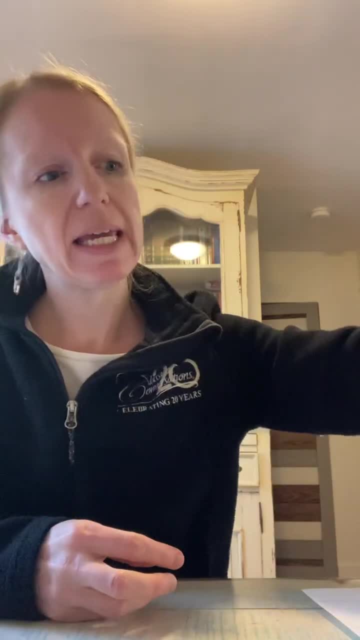 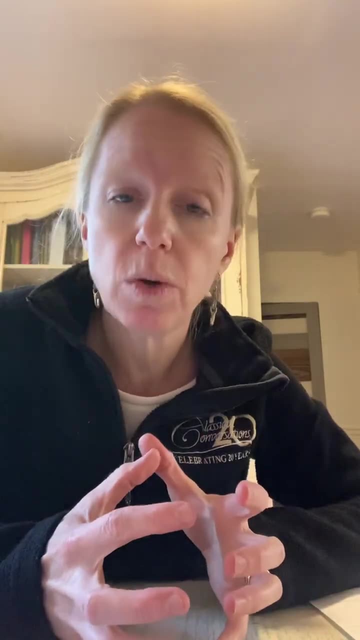 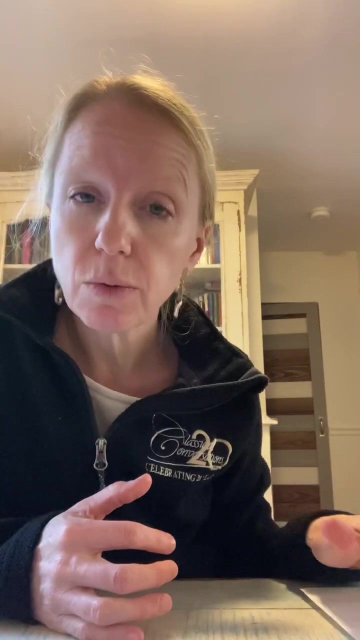 So kind of a summary of that. we are taking a sample, We're taking about a fourth of the total number of chips in here And out of that sample we are making a conclusion or a probability estimate about the whole group. We're saying, based on our sample of 25 draws, there's about this percentage.